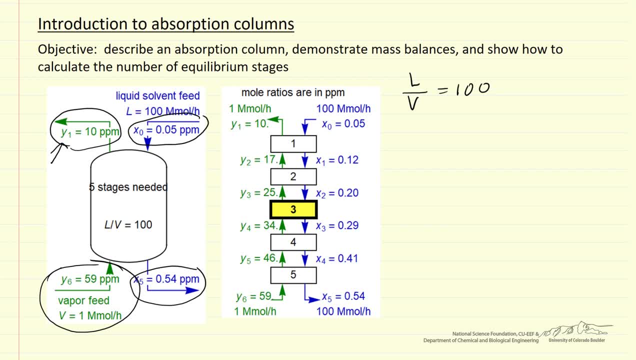 so they're very close to mole fraction because the concentration of solute is really quite low. So if we look at a column with five stages, you can see that the concentration 59, in the gas phase decreases with each stage, whereas the concentration 0.05, in the liquid phase. 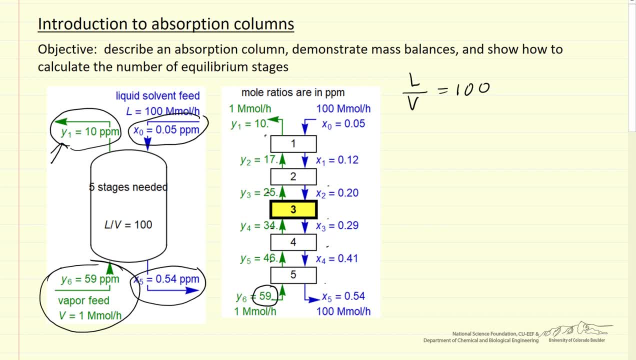 increases with each stage. Now notice this corresponds to 59 mole per hour being fed of the solute and we multiply by 10 to the sixth, And this corresponds- because the flow rate is a hundred times higher- 54 moles per hour to solute. So we're removing approximately 95% of the solute, that's in. 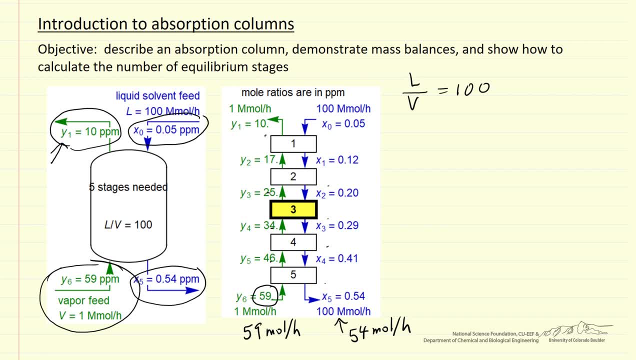 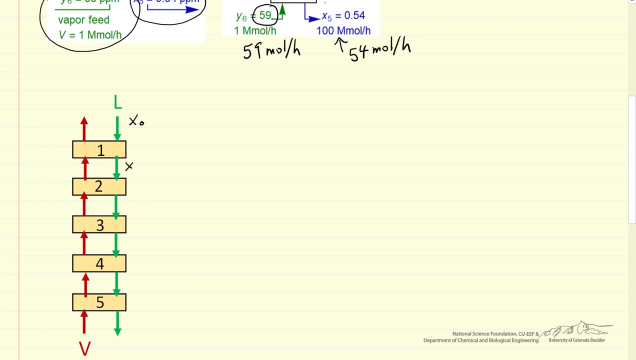 the vapor phase. So let's look at the mass balances that we use to analyze this type. So, on this diagram for mass balances, we'll call this X, zero, and then mole fraction or mole ratio in liquid phase. the subscript corresponds to the stage that it's leaving. 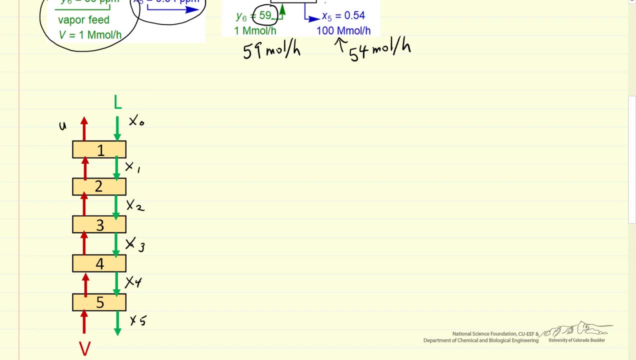 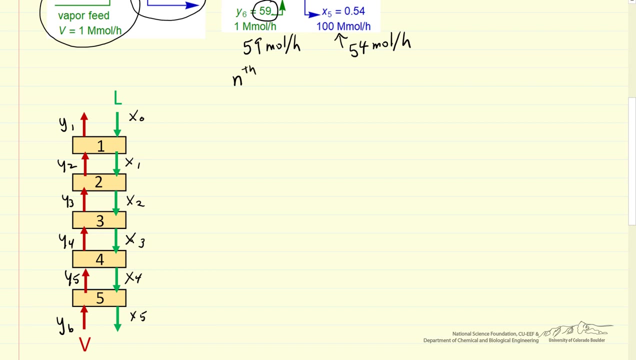 And likewise for the vapor phase the subscript. so we'll use Y vapor phase mole ratio. the subscript corresponds to the phase that is leaving, which means this is Y six. So if we look at the nth stage, then the mole ratios leaving X, n and Y n. 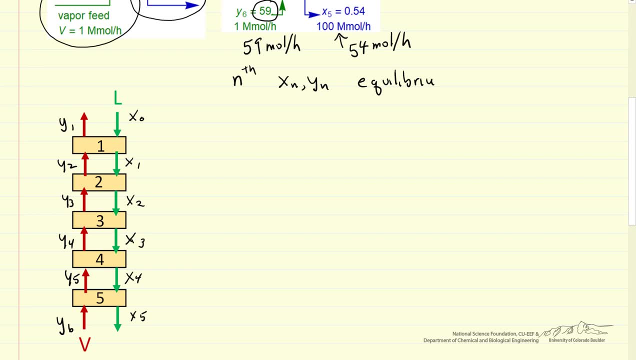 these values are in equilibrium. That's what we're assuming in this analysis. Because such low concentrations, parts per million in this case? we will model this by Henry's law and say: Y, n is equal to Henry's law. constant over pressure times: X, n. 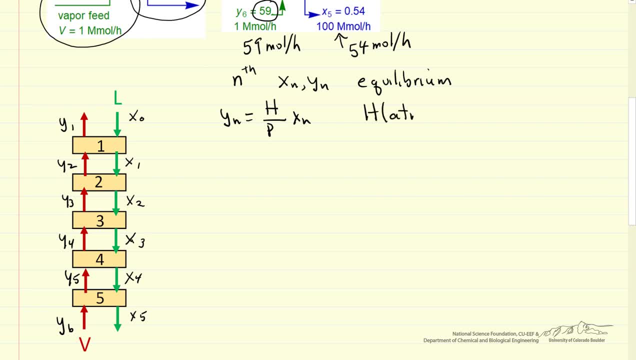 So Henry's law constant in this case has units of pressure. There are different ways defining Henry's law constant, And so let's look at a mass balance for this part of the system And, if we're gonna do now, a mass balance on the solute. 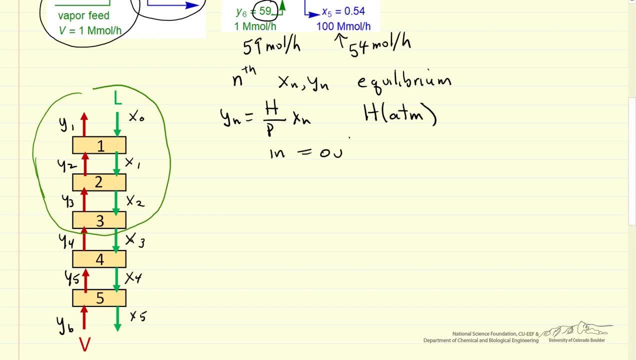 we're essentially saying solute flow in equals solute flow out. Flow in is X zero times liquid rate, plus Y four times the vapor flow rate, And what's leaving then is X three liquid flow rate plus Y one the vapor flow rate. 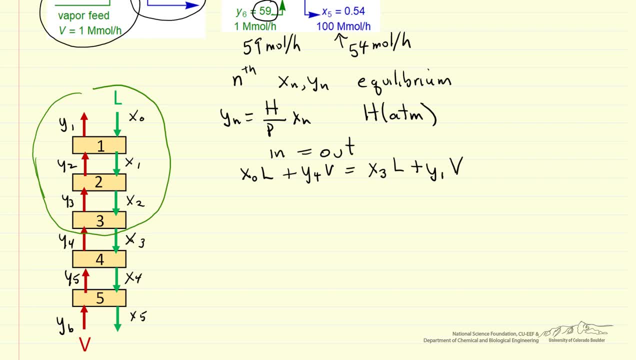 We can do a balance for any number of stages, just one and two or all five, And so the general form of this equation is Y n plus one, Because, remember, this was stage three, X n times L plus Y one. Remember, we have the first step here. 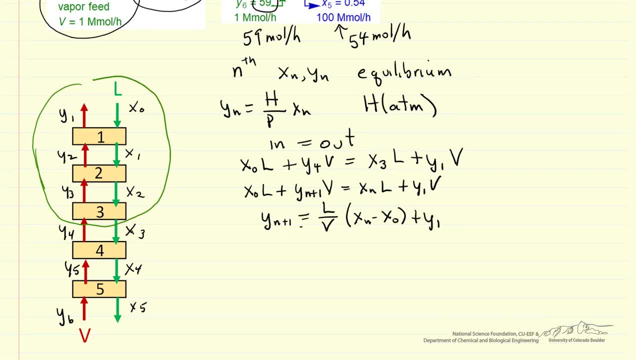 1 times v. So that's just a rearranged equation and this is what we're going to call the operating line. And so if we want to determine the number of stages, we're going to plot the operating line and the equilibrium line and then we'll step through how we do that calculation to determine the number. 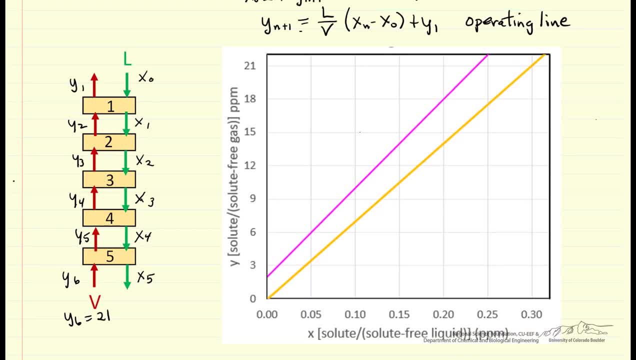 of stages. So I'll plot some example values. This is the equilibrium line, Henry's Law, so it's linear. This is the mass balance line, the operating line, and that's this equation. here And I picked a value for y6 of 21.. So that has to be on the mass balance line and the way we determine. 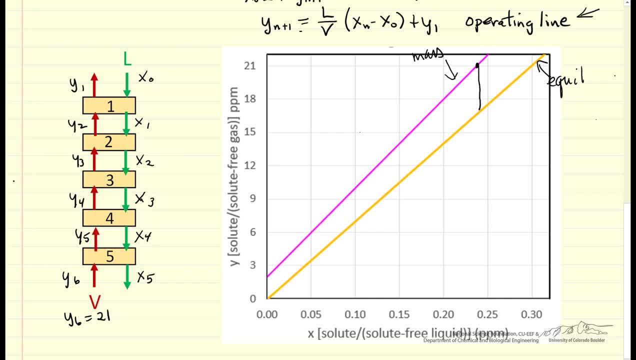 equilibrium stages is that if this value here is y6, this value then is going to be y5 and x5.. Because x5 and y5 aren't equal, x5 is equal. So this line is the equilibrium line. This is the equilibrium. 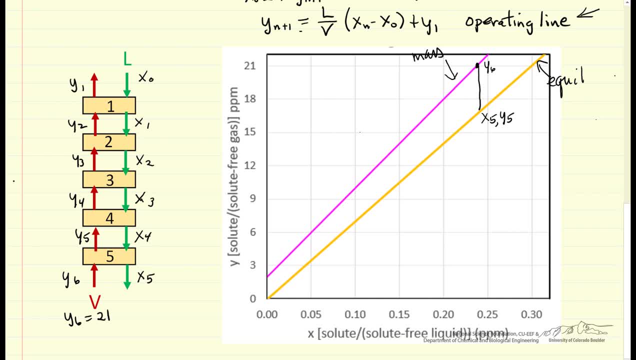 The values leaving stage five have to be in equilibrium, so they need to be on the equilibrium line. Well then, for the mass balance, this point is x four and y five, because x four and y five, you can see, here is where we do a mass balance. 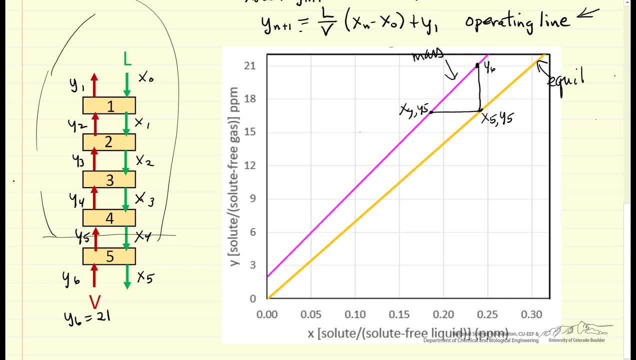 We do say a mass balance around this. They have to satisfy the equation and we can step through. This is still x four, but now it's y four and of course x four and y four, leaving stage four, have to be in equilibrium. 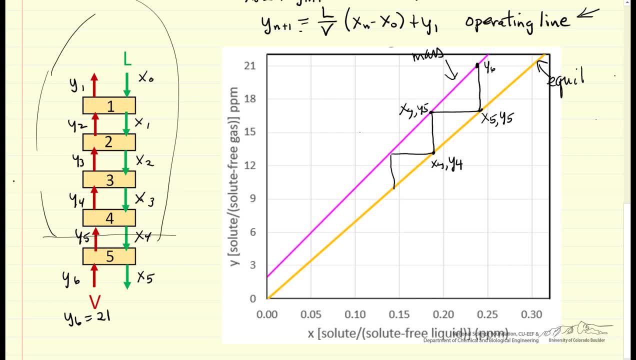 and we can continue. and doing this by hand, of course, is not as accurate as if I was a little more careful, but I can do this until here is x zero. We don't have another stage. Here is x zero because that's what has to be on the mass balance line.